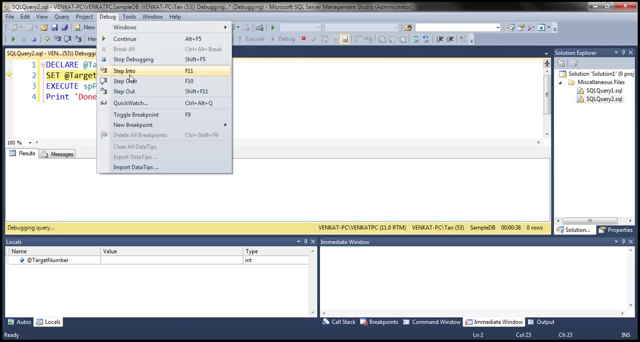 whether you choose step over or step into, it doesn't really matter. Let's choose step over. Now the debugger is about to execute line number three. Here we are calling a stored procedure, as we print even numbers. So on this line, if we use step over, then the debugger will not. 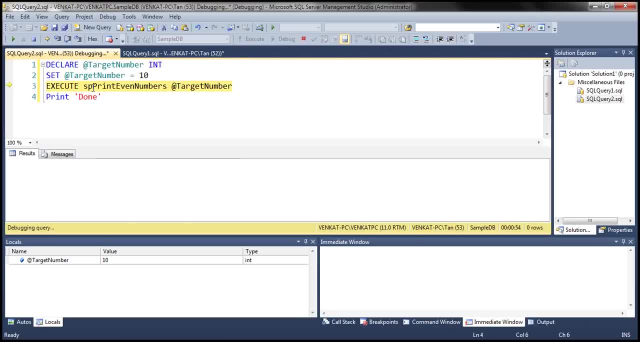 provide us the opportunity to debug the stored procedure line by line. This line will be executed in its entirety. Let's look at that, Look at this. When I select step over, it didn't actually step procedure line by line. Now let's continue debugging and let's start the debugger once. 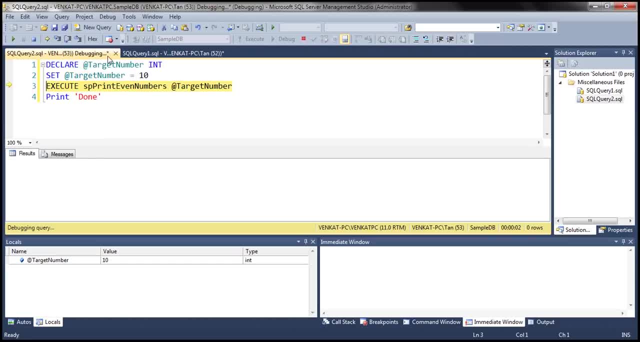 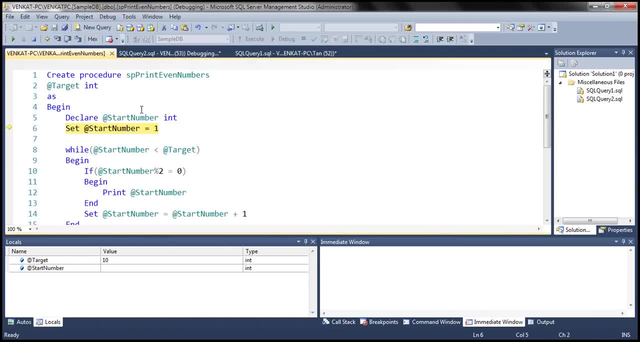 again and let's choose step over. Now, on this line, instead of using step over, I'm going to select step into. So when we selected step into, the debugger has actually provided us the opportunity to debug this stored procedure line by line. So now I could use either step over or 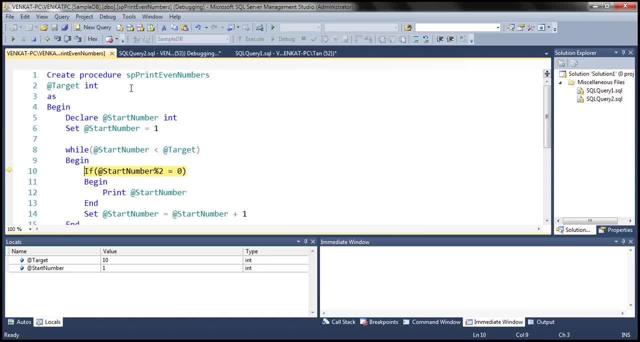 step into and debug each line of this stored procedure. So what is step out then? Now we are debugging within the stored procedure. Now, for some reason, at this point I have realized that the problem is not within the stored procedure. So I want to step out of the stored. 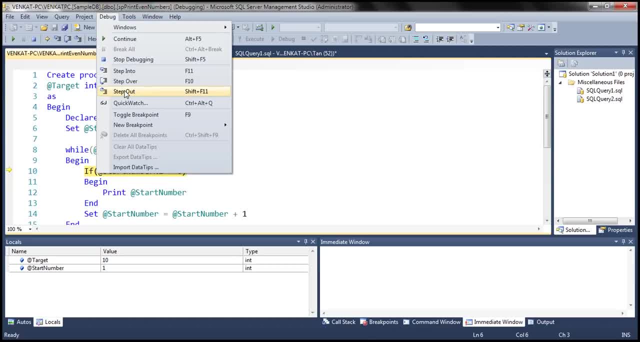 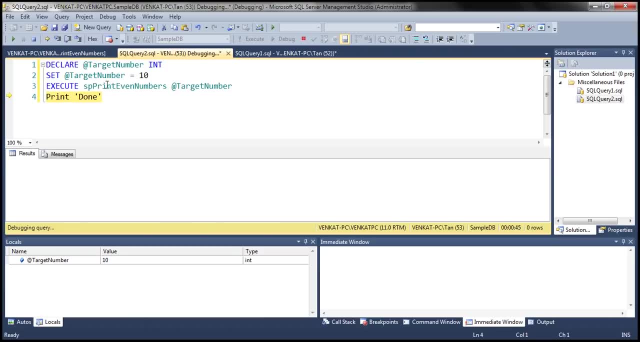 procedure. That's when we use step out. Let's actually select that option and see what's going to happen. Look at that: The debugger has finished executing that stored procedure and it's waiting on the next line, That is, on line number 4 right here. So that's what these three options does: Step into step. 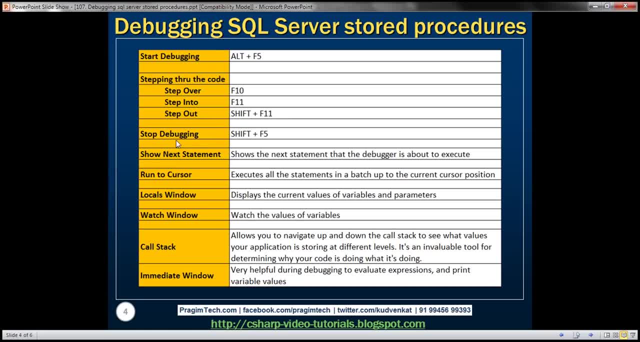 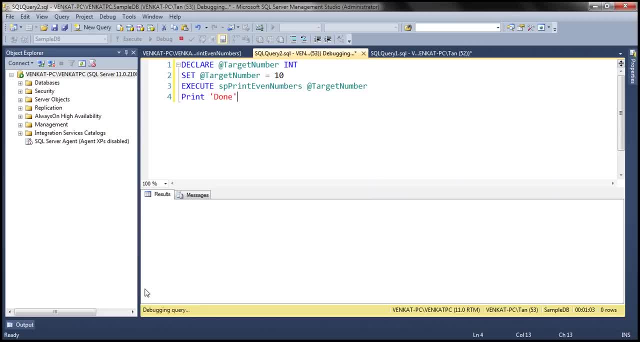 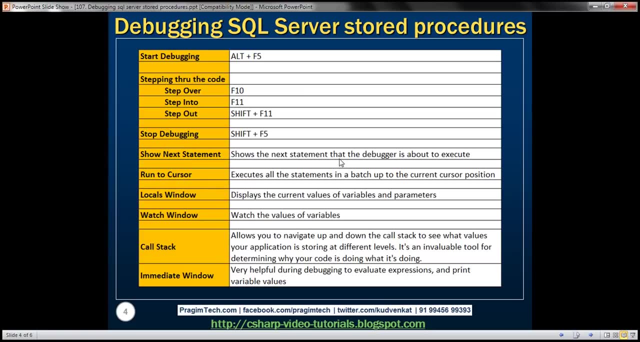 over and step out. To stop debugging, we can either use shift F5 or, from the debug menu, select stop debugging. Show next statement. This command is useful to show the next statement that the debugger is about to execute. This is extremely useful when you have several query editors window. 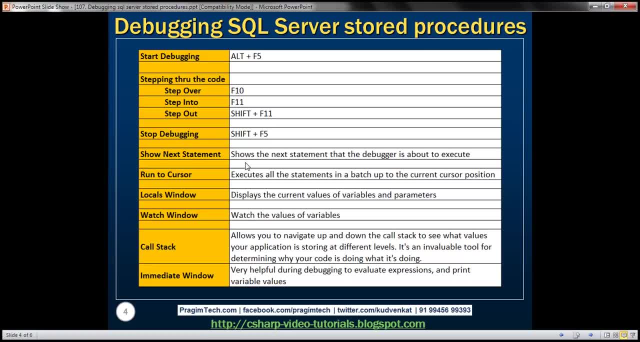 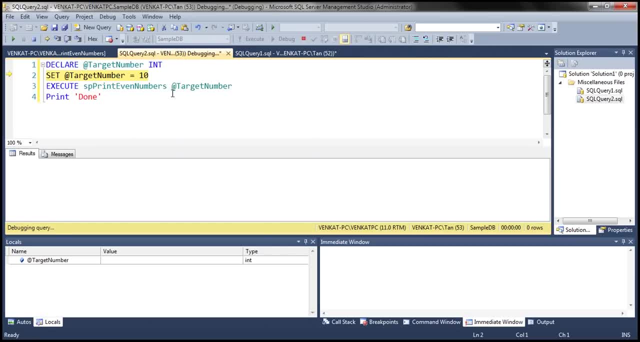 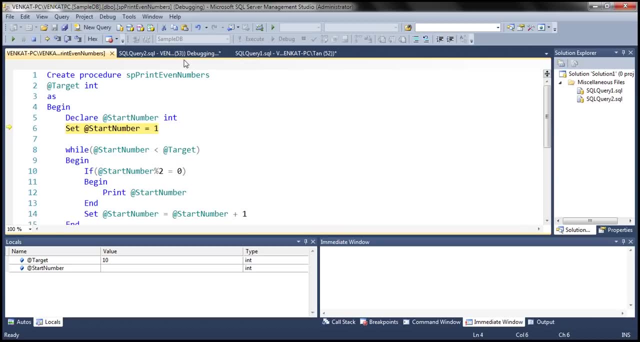 open and you don't have to do anything else. So let's start the debugger. So let's start the debugger once again and let's actually step over and then step into executing the stored procedure. Now let's say we have several windows open here. Now I don't know where the debugger. 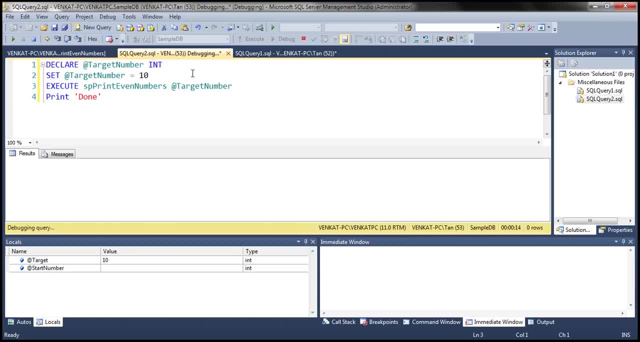 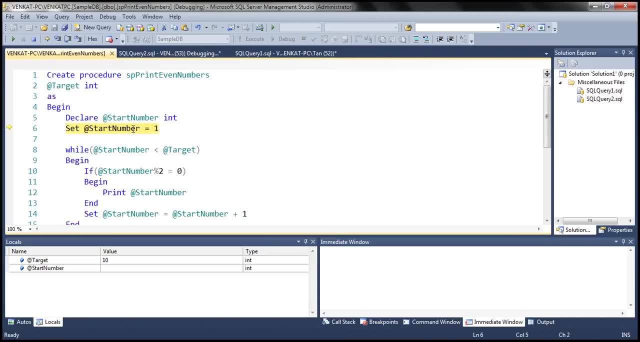 is At this point. if I want to see what is the line that the debugger is about to execute, I can simply right click and then select this option. show next statement. Now this is going to take me to the file that the debugger is about to execute, which is very useful. Run to cursor This command. 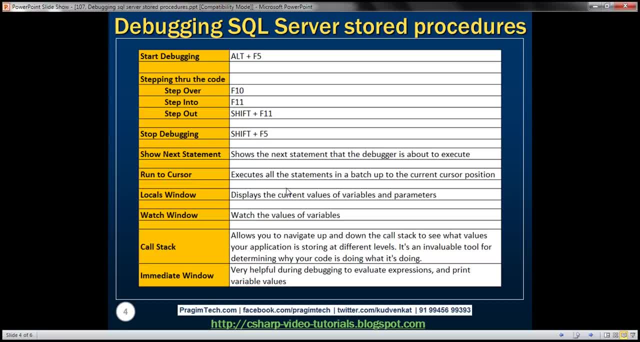 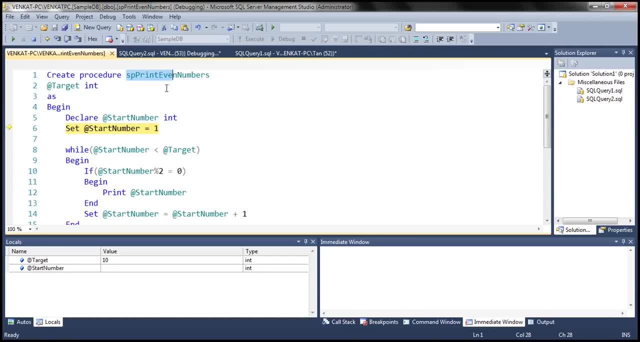 executes all the statements in a batch up to the current cursor position- Again, very useful. Let's actually look at that with an example. Look at this: right here We are within the stored procedure, debugging, and we have a while loop here, right? So I am debugging the while loop, Since this is a 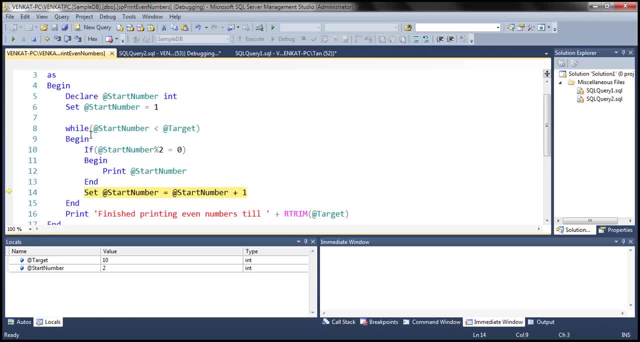 loop. you know it's going to be stuck inside this loop until this condition becomes false. Now let's is that? the problem that I'm trying to solve is not within this loop, So there's no point wasting in time executing you know, this while loop until this condition becomes false. Now I actually want. 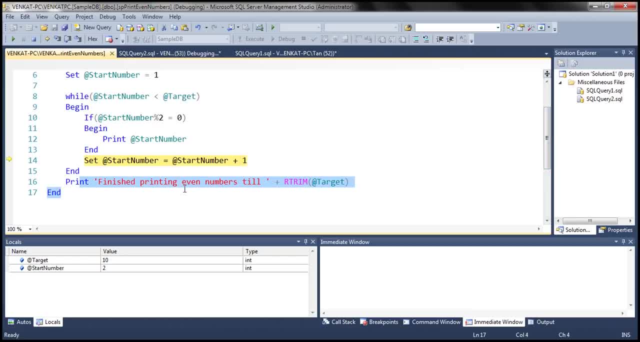 to see what happens when this line is executed. right, So I want the cursor to run that to that line. Okay, so what I can do is right click on that line and then select this option: run to cursor. So what is the debug going to do? It's going to execute all this code in the while loop And then 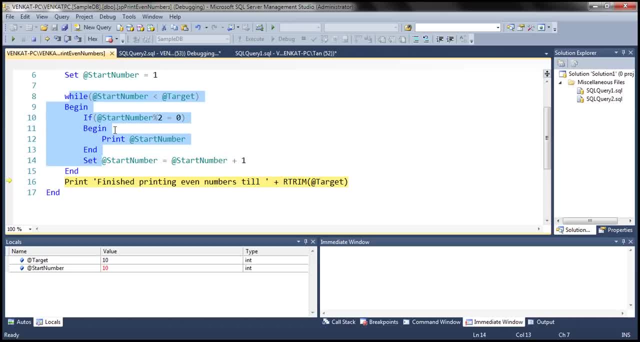 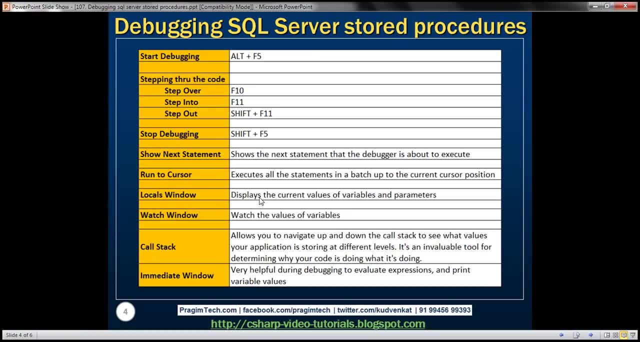 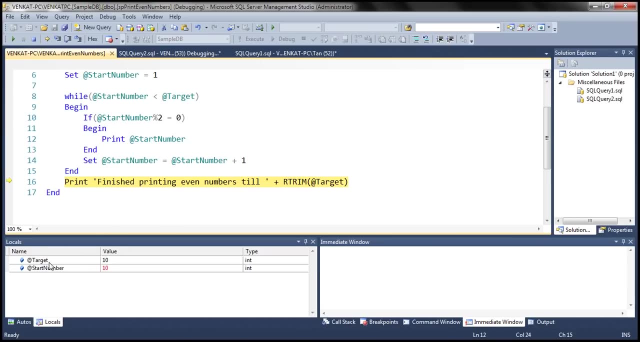 it's going to come right there, So it's going to save a lot of time. So that's what run to cursor does: Locals window. this window displays the current values of variables and parameters. So let's go to SQL Server Management Studio. Here we have the locals window And look at this At the 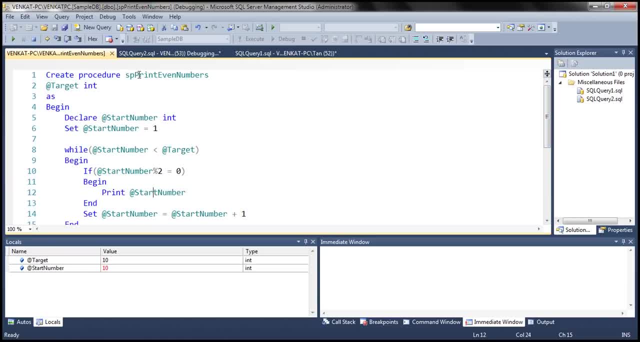 moment we are within the context of this stored procedure, has been print even numbers And if you look at this stored procedure, we have the current values of variables and parameters. And if you look at this stored procedure, it has got an input parameter and a local variable start number. So 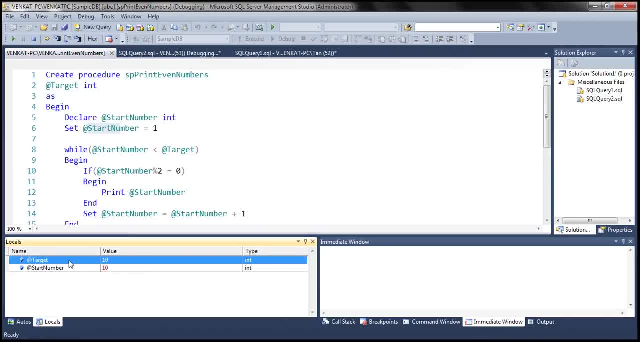 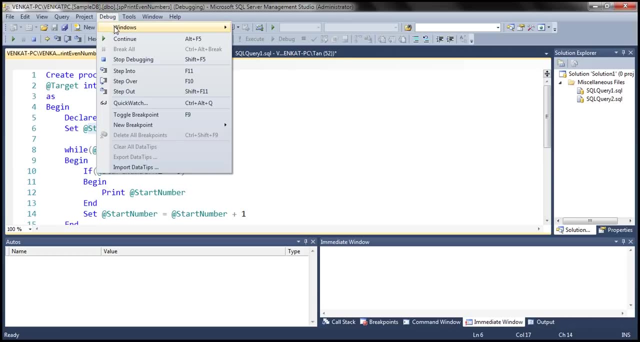 target parameter: its name, its value and its data type. Similarly, start number variable: its value, its data type. So that's what the locals vendor does. Now let's say you have closed the locals window. Now you want to bring it back. it's actually present in debug menu: vendors and 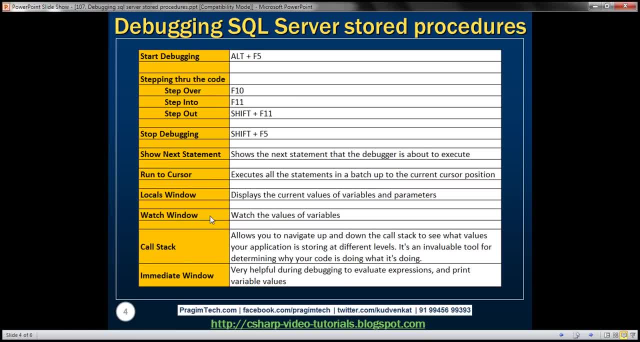 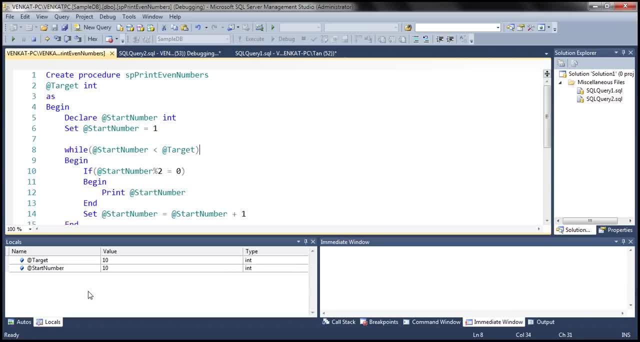 locals Watch window. this window is similar to locals but it's actually present in debug menu, similar to locals window, which is used to watch the values of variables. Now, if you want to add a variable to a watch window, simply select that variable, right click on that and select add to. 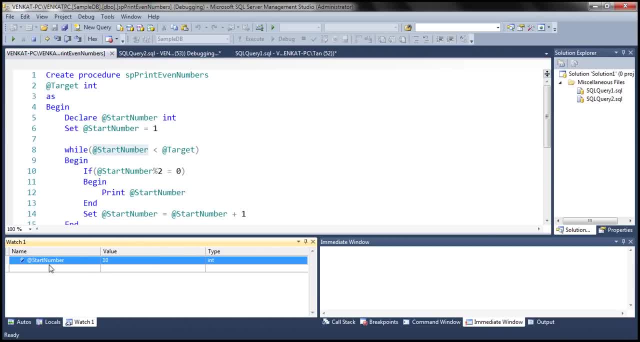 watch. So this variable is added to the watch window. look at this watch window also display you know similar data name of the variable value and its data type. Now if you want to add a different variable to watch window, select that and add it to the watch window. Okay. 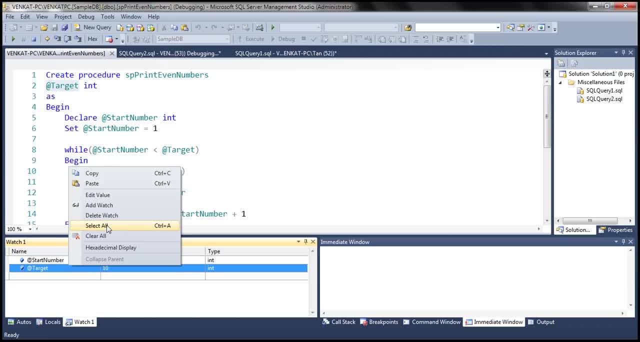 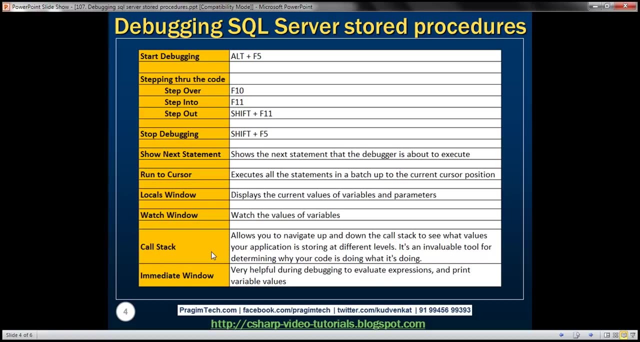 now. if you want to delete a variable, simply right click on that and select delete- watch. If you want to remove all of the variables, clear all. So watch window. very similar to locals window, Call stack. this allows you to navigate up and down the call stack to see what values your application is. 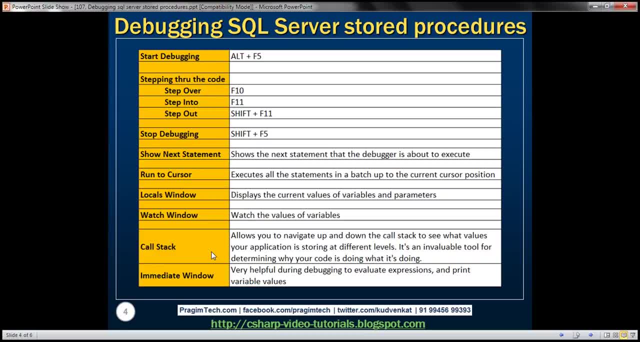 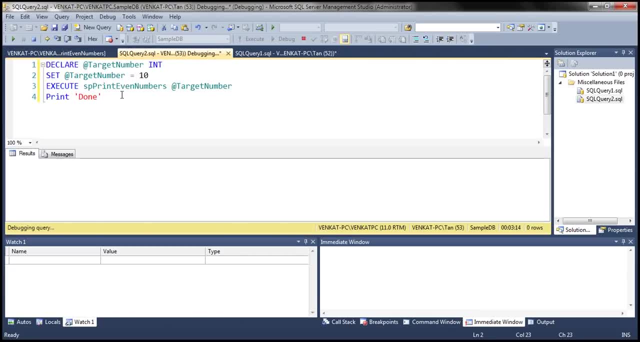 storing at different levels. It's an invaluable tool for determining what your code is doing, what it's doing at the moment. Let's actually understand this with an example. Now. this is the main query editor window, sqlquery2.sql, where we have our transact sql code. 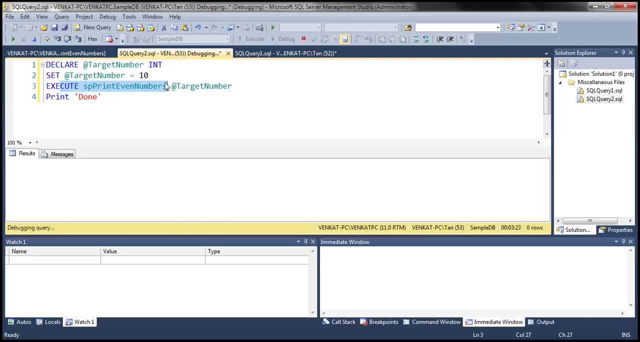 where the debugging started And this actually called SP. print even numbers And to get your call stack window. it's right here, Notice, within the call stack window we have our sqlquery2.sql. Now if I double click on that it takes me to the window which called that stored procedure. 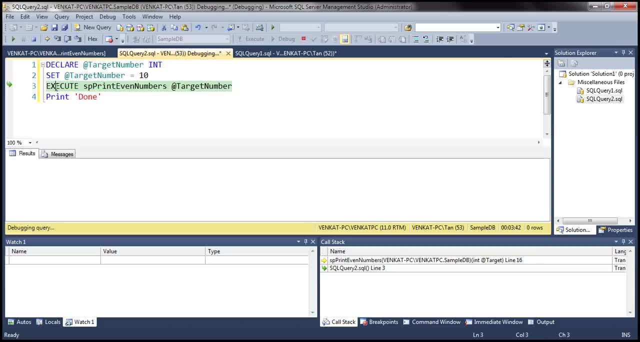 SP print even numbers. Look at that. within that window, the line which called stored procedures highlighted in green, and within our locals window I can actually see, at the time when that stored procedure is called, what is the value of this variable target number. 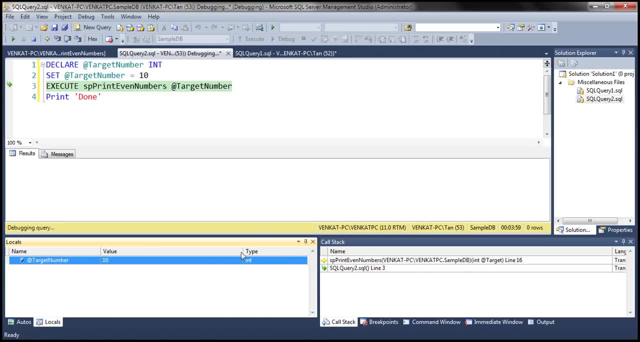 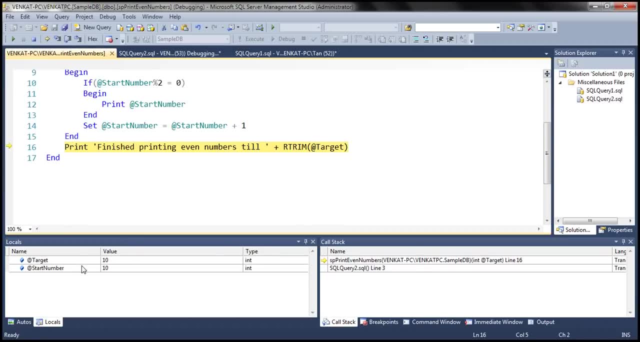 its name, its value and its data type. And now, when we change the context to the stored procedure, look at that. the locals window shows the variables names, the values and data types And here the call stack is showing us who is calling what. 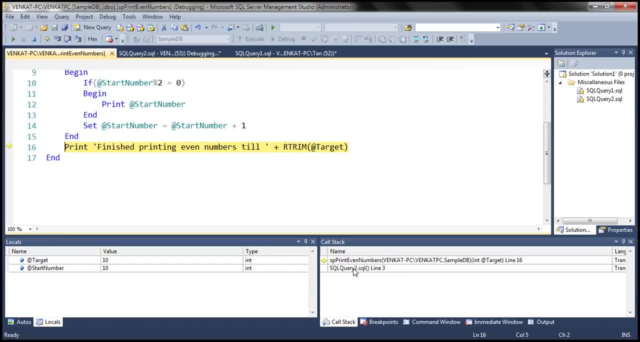 what? what are their values when those calls are made? At the moment, you know we only have two windows, but imagine a situation where you have a stored procedure calling another stored procedure, that stored procedure calling another stored procedure and that stored procedure calling another function. So you want to see who is calling what. what. 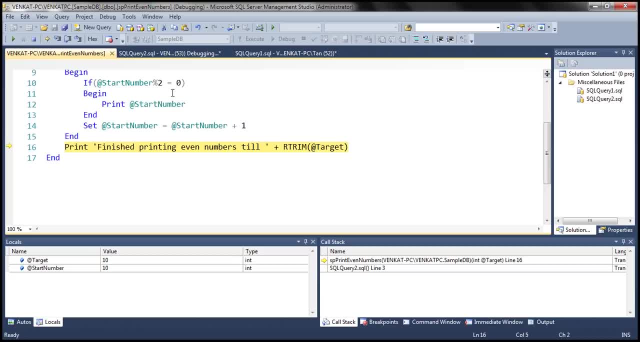 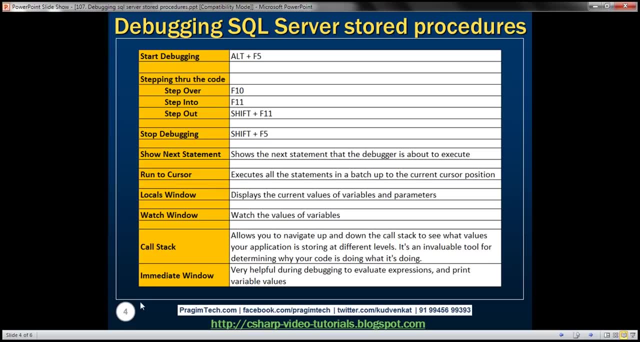 are the values of variables and parameters at these times. you know you can use call stack, which is extremely useful for debugging and figuring out what's going wrong. Immediate window: this is helpful during debugging to evaluate expressions and print variable values And to get to the immediate window. it's right here and we can use this. 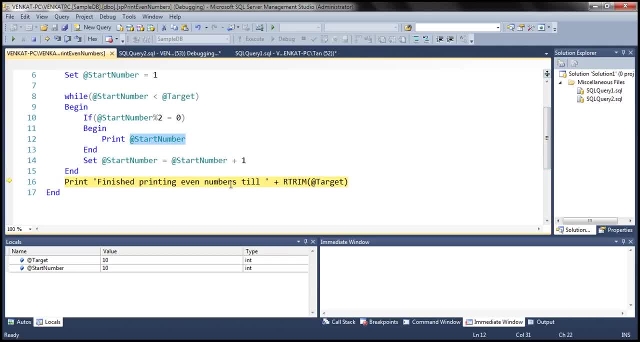 to print variable values. So here we have a variable start number. If I want to see its value, I simply type it here, press enter. so start number value is 10 at the moment. I can also evaluate an expression here. So I want to see what value I get when I divide. 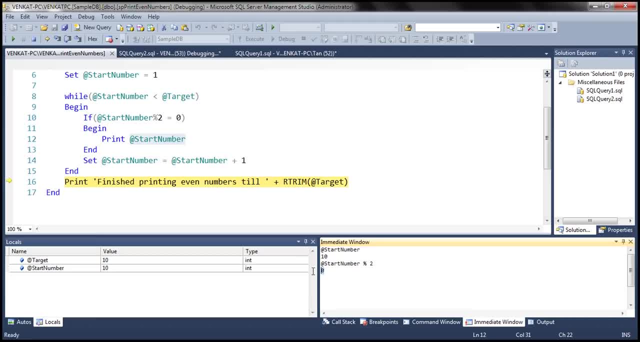 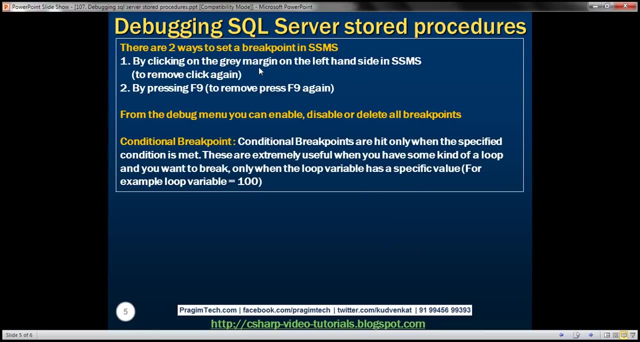 start number by 2, the reminder is 0.. If you want to clear the contents of immediate window, simply type angular bracket followed by CLS and press enter. That's going to clear the immediate window. Now let's turn our attention to breakpoints. There are two ways to set breakpoints in SQL. 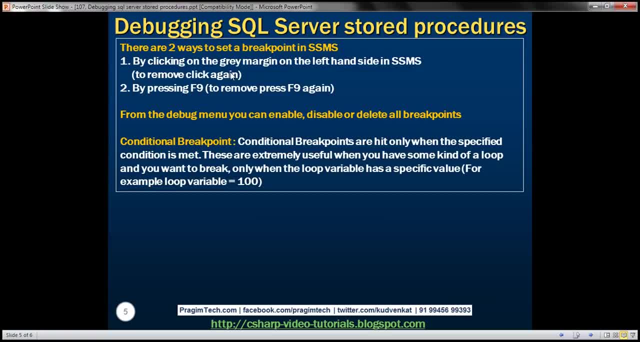 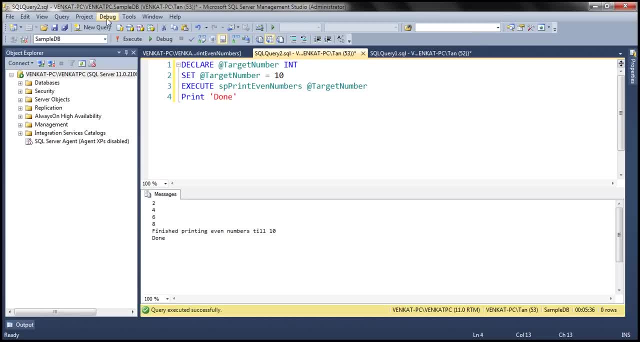 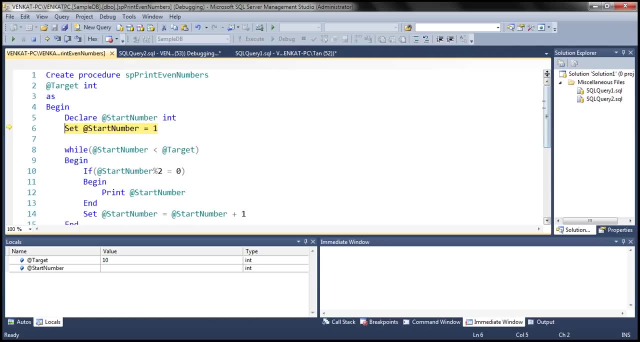 Server Management Studio. You can do that either by clicking on the grey margin on the left-hand side in SQL Server Management Studio. Let's actually continue and let's start debugging once again And let's step into executing. Let's start the procedure Now. I can set a breakpoint on this line if I want to simply. 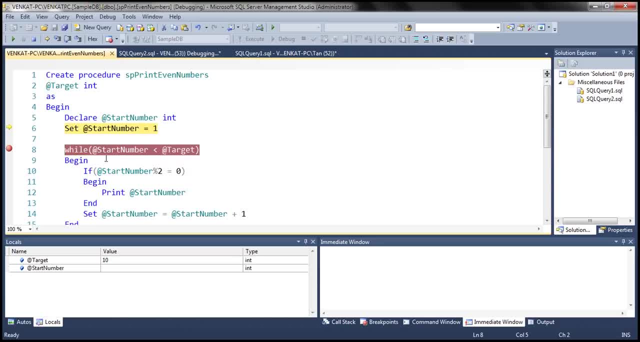 by clicking on the grey margin right here, or I can use the keyboard shortcut F9.. F9 is actually going to toggle the breakpoint. If the breakpoint is already there, it's going to remove that. If it's not there, it's going to set that. Look at this when I press F9,. 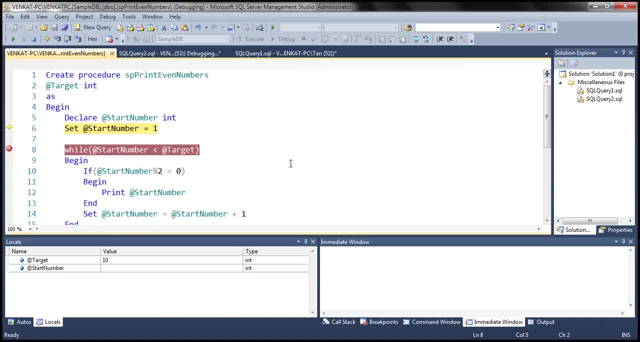 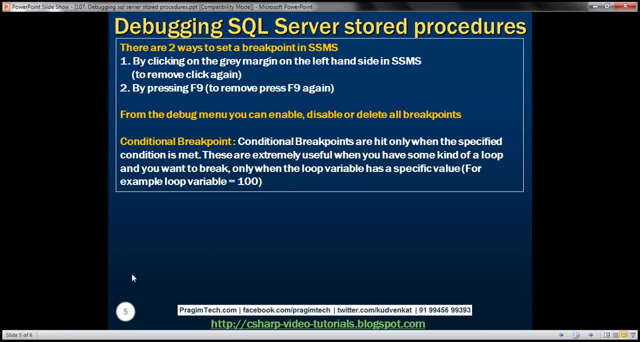 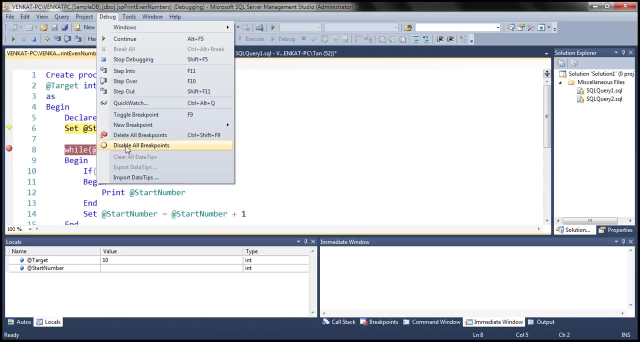 it toggles the breakpoint. Now you also have the option to enable, disable or delete all breakpoints at once, And you can find those options in the debug menu. Now let's say I want to disable all breakpoints that I have set. I can select this option. Look at that. 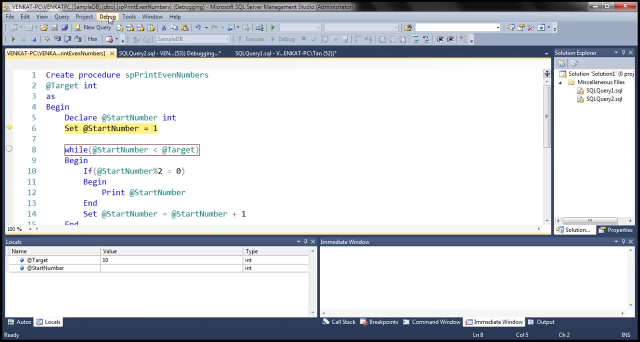 When I disable a breakpoint, that's how they look like And if I want to enable them back, I can come and select this option. If I want to delete all the breakpoints, we can select delete all breakpoints And at that point it's going to throw this confirmation Do. 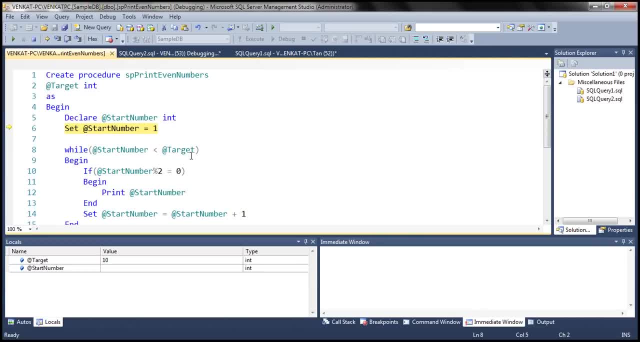 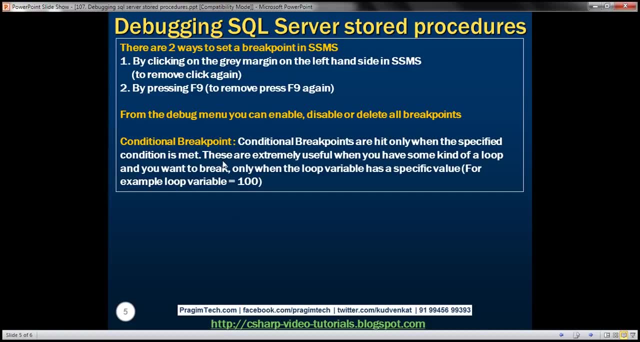 you want to delete all breakpoints. When you click S, it's going to delete all the breakpoints. Conditional breakpoints are hit only when the specified condition is met. These are extremely useful when you have some kind of a loop and you want to break only when the 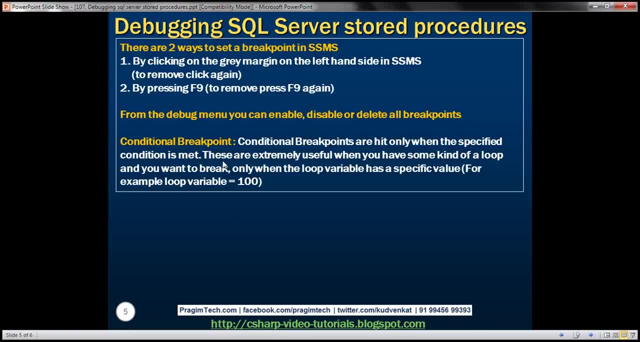 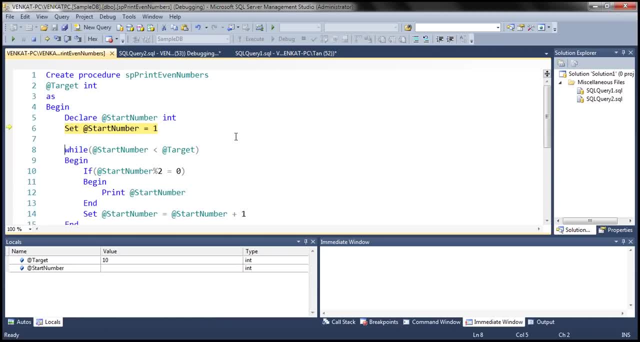 loop variable has a specific value, For example, when the loop variable is equal to 100.. Let's actually understand this conditional breakpoint, because this is very helpful in debugging. Now, here we have a while loop And obviously when I throw in a breakpoint right here and 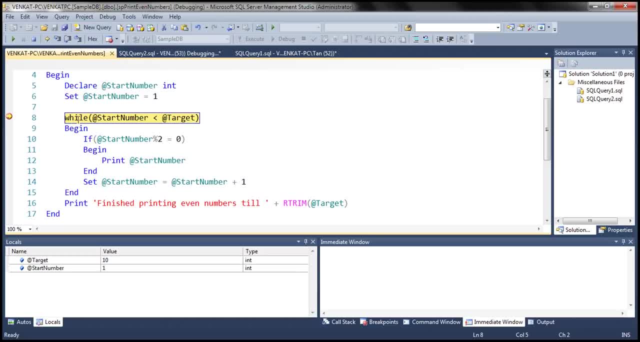 when I select continue, it's going to be hit right. This breakpoint will be hit every time. you know, the code comes to that point. So at the moment, start number variable has a value of 1.. Now I want. 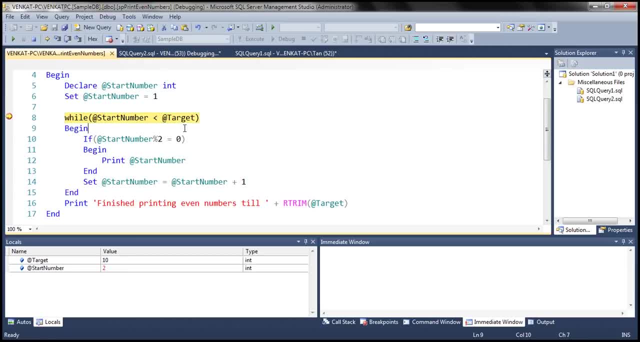 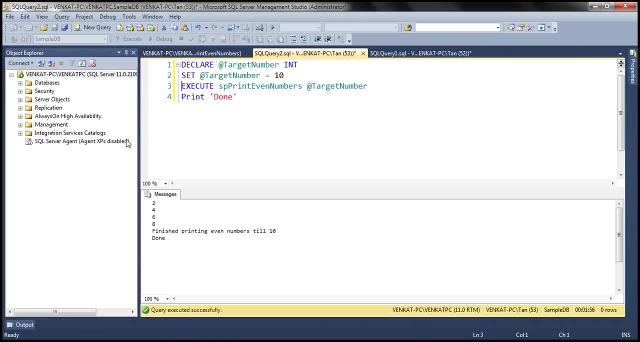 to continue. Start number variable is 2.. Now, actually, let's disable that breakpoint and let's continue So it finishes. And look at this: This stored procedure at the moment has got two problems: It doesn't start from zero and it doesn't. 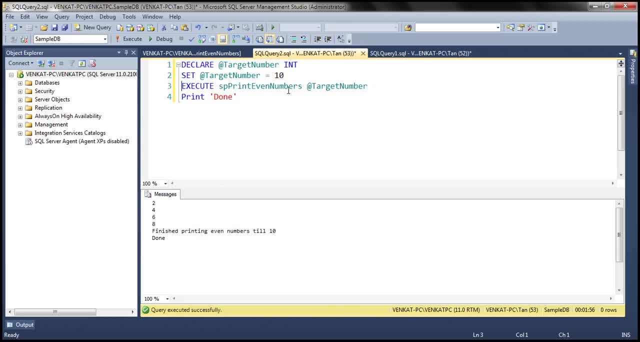 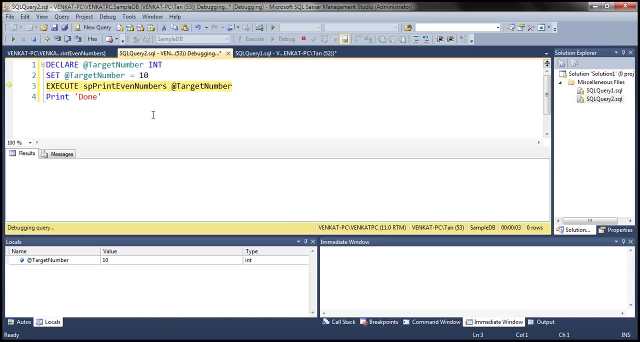 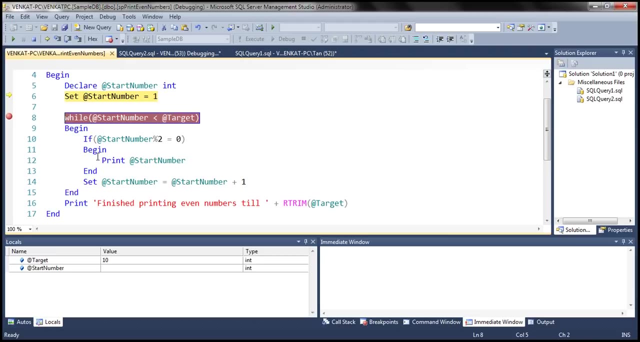 print till 10, right? So let's see where the problem is by debugging it. So I'm going to start the debugger and I'm going to press F10 and then F11 to step into that stored procedure, and I'm going to enable this breakpoint simply by clicking on that Now when I press. 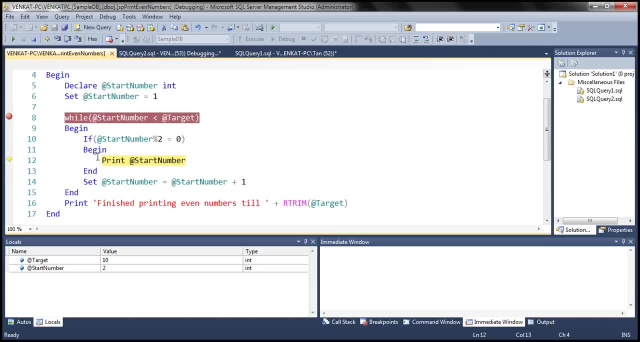 F10 and when that breakpoint is hit, or when I select Alt F5, you know, notice this breakpoint is hit every time and I don't want that Because you know what is the problem with this stored procedure? It's not printing zero. 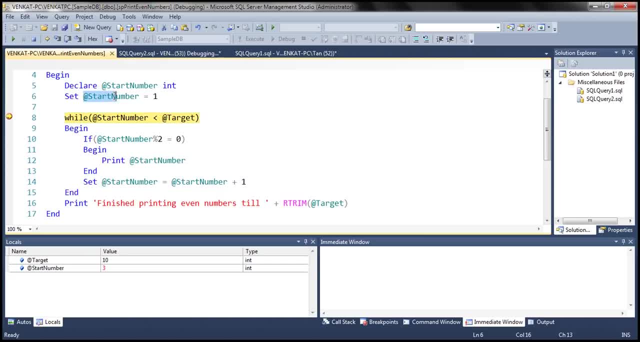 and that could possibly be because we are starting this counter at 1 instead of zero. We know that first problem. But the second problem is you know it could be right here, because you know it's printing even numbers until 8, okay, And after 8, it's not printing. 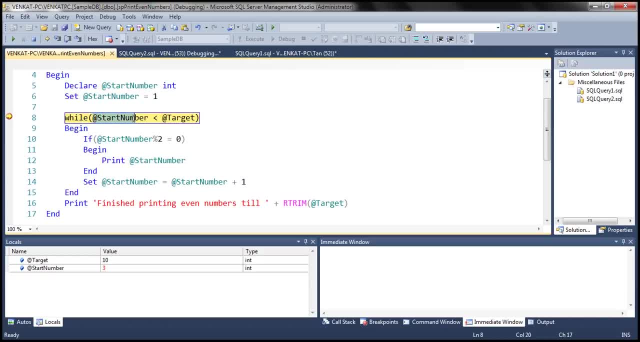 10.. So as long as this variable value is 8, it's getting inside this loop and it's doing what it is supposed to do. Subtitles by the Amaraorg community. But when it becomes, you know, greater than 8, maybe that's when the problem is. So I 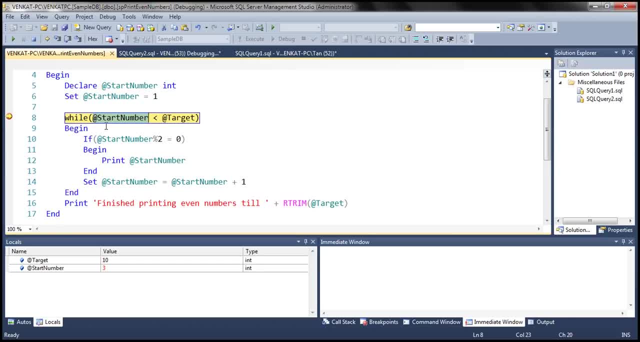 want this breakpoint to be hit only when this variable value is greater than 8,? okay, But at the moment, since we don't have a condition on that breakpoint, it will be hit every time. okay, So to make this a conditional breakpoint, all you have to do is simply right-click on.